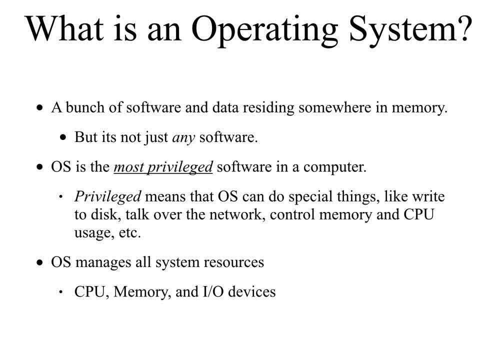 software can run on the CPU, for how long and when. So, essentially, operating system can do special things that deal with allocation and control of a computer systems resources which other normal software are not allowed to do. So broadly, these three resources, we can categorize them as CPU memory and IO devices, or input output devices. 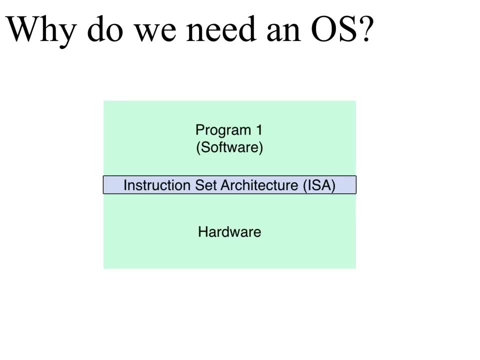 So one might very reasonably ask why one needs an operating system in the first place. If we have a computer and its hardware resources available, then why can't we just run any program we want directly on the hardware and let it directly manage the hardware resources? So normally if you take a computer's hardware resources- the CPU memory and IO devices- these are accessible to any software. 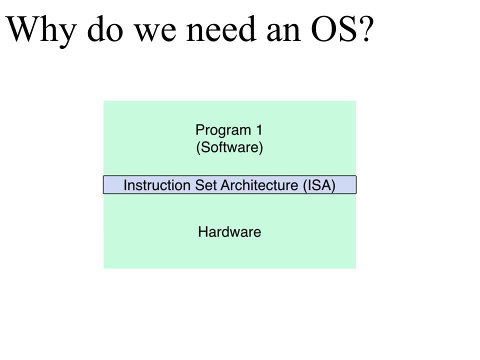 running on the computer through an interface which is the hardware software interface. the hardware software interface has a specific name. it's called the instruction set architecture. Instruction set architecture: you can think of it as the set of instructions that a software can issue to the CPU, using which the CPU can then initiate actions to control various hardware resources. Now, 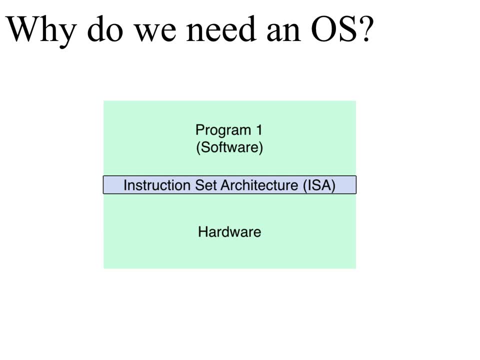 any interaction between software and hardware happens through these ISA, and ISA is defined by the hardware vendor, such as, say, Intel or AMD. so if you essentially have a software that can directly run on the hardware, meaning it can issue instructions directly to the hardware, then why can't that? why isn't? 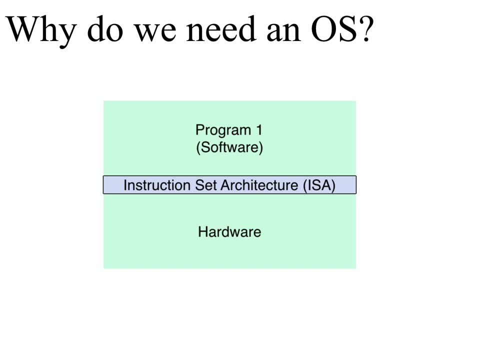 that enough like. why do you need a special piece of software called OS to interject itself between your application and the hardware? so a, if you want, this is certainly possible. if your program was the only program running on the computer and it, it knew exactly what it was doing, how to communicate with the 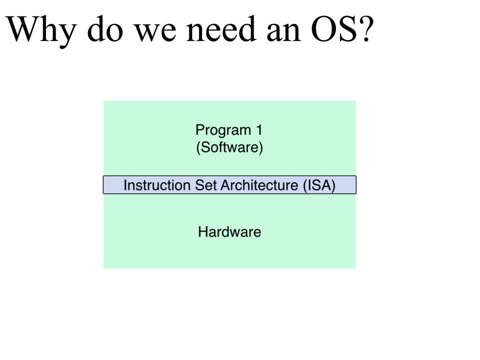 hardware. you could certainly do something like this and many times when you don't want additional overhead, certain embedded systems, for example, might be designed to run a custom design software for a specific hardware to do a very specific task. more often, regular user level programs don't know how to talk to the underlying 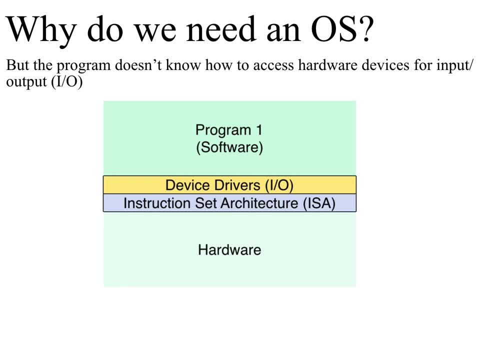 hardware. there are various types of hardware with various peculiarities. there are various types of CPUs, various types of memory controllers, various types of disk controllers and so forth, and it is almost impossible for any single program to run a custom design software for a specific hardware to do a very specific task. 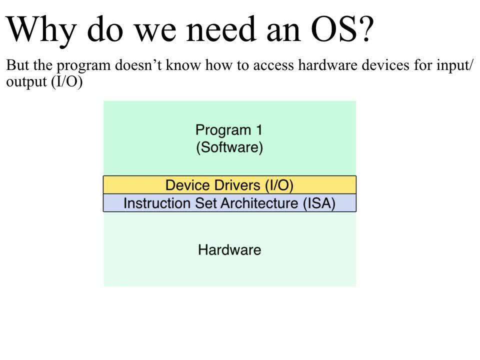 and it is also impossible for any member of the Hardwareare software to do a very specific task for an extended branch, kind of, at the domain of libraries that are actually being used. it can be any malware. software can run on MSP, for instance. so what's a potential property of raw hardware? 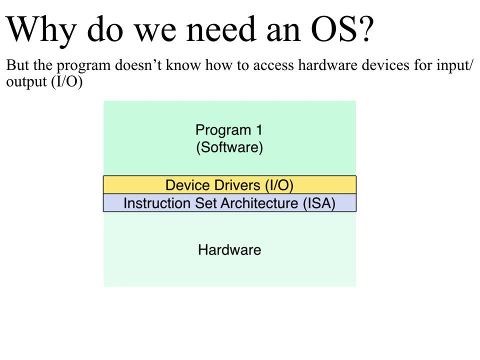 to run a custom design software on freeимер hardware in the near future. well, actually, in effect it could be anything. it's anno go. I will have to pause quickly and do some Arkani by itself in a minute. we'll do some Porki drivers and then, once that's done, you could run the resulting binary directly. 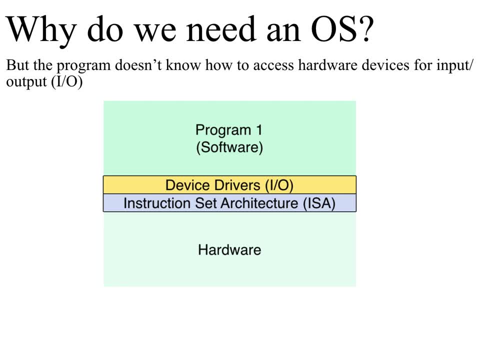 on the hardware right. so now we have begun to introduce aspects of modern operating system into into this picture between the user program and the hardware right. but if this was the only program to run on a given hardware, then it could link the necessary device drivers and happily have direct access. 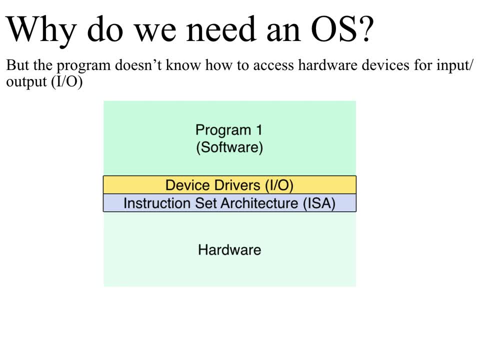 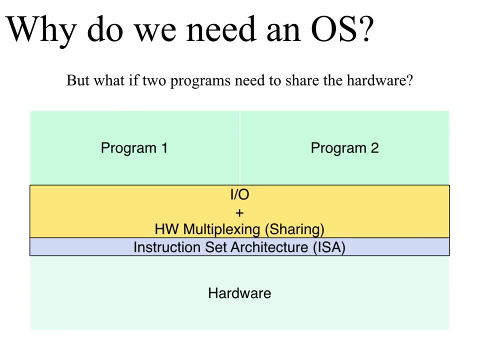 to the hardware without any additional OS support. however, now let's consider a situation where we want to run more than one program on a given set of hardware. what that means is these two programs have to share the CPU, share the memory and possibly share the IO devices. 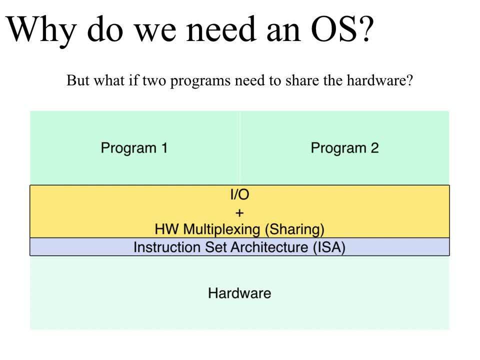 you. so the question is, you know, do we just rely on these programs to be nice to each other, or do we want some other additional piece of software to arbitrate between these two, to have them executing nicely without interfering with each other? so now we can add some additional software for multiplexing, for 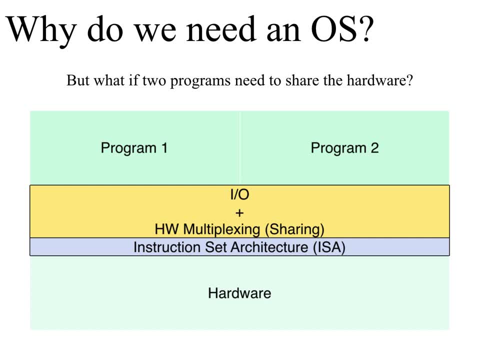 hardware multiplexing, or in other words, hardware sharing, because you see, this is a broad story- into the, the network card and so forth. so now, as you can see, we are buildinng scheduling, green and resource allocation into this integral program, which is what this and this looks like very short and very short. but what now? what is this? it JFPSность is that in addition to the Dr on that, the other. so now it you can get it on that drive drive we saw in the previous slide. now we need some other software compet entra. so what do we need to do? if we can get ability software component to do this? two, the programs get to run on the hardware at any given time on the CPU and get to run on the hardware which part of memory they can access. then they can access when they can access the hard. diskash sets harddisk aside, altro cardfilers at the same time. so now, as you can see, we are building scheduling green resource allocation. now, as you can see, we are building scheduling resource allocation. 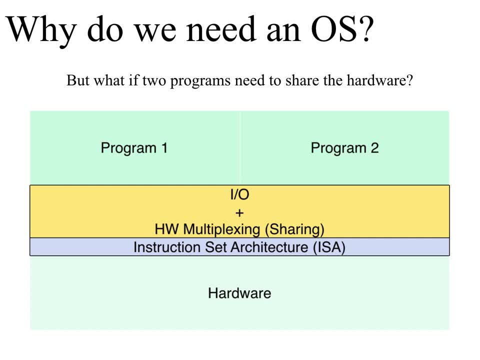 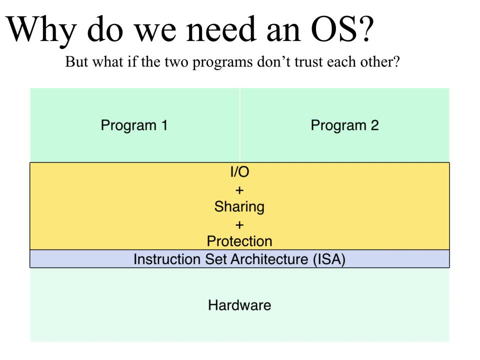 software, which is which now looks more like traditional operating systems. now, within this picture, assume for a moment that the two programs that are going to share this hardware, they don't trust each other and they are mutually untrusting or they can be potentially malicious. so we need some additional. 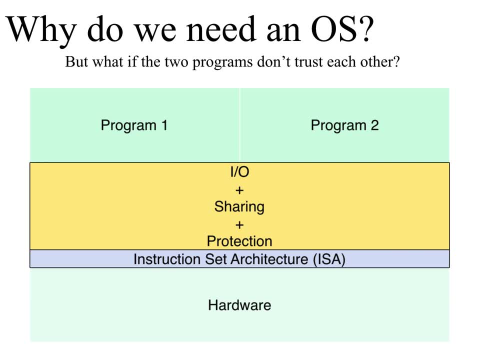 software that can enforce protection, meaning that it can protect one program from another program running on the same machine sharing the same hardware. so in addition to having device drivers for IO and sharing or multiplexing mechanism for resource allocation, we need some protection mechanism to prevent illegal 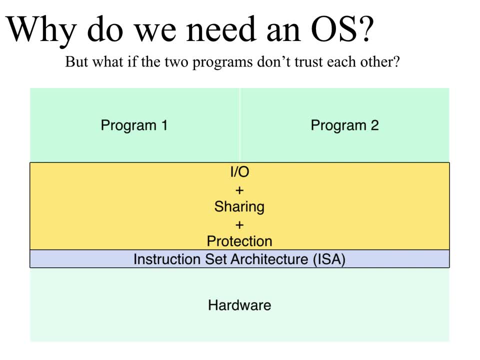 or unauthorized access to data and IO devices by you, one program or the other program. so there are various types of prediction models, are what are also known as, more formally, threat models that one may have to consider. of course, protecting one program from another is really important between, say, mutually untrusting users, but it's also important now that this 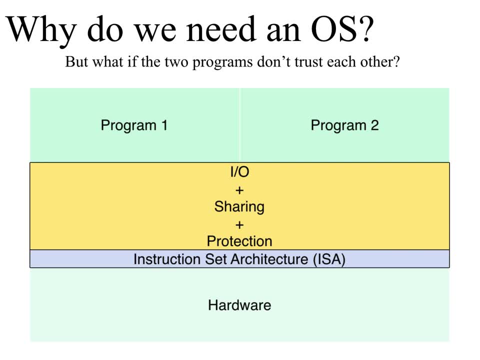 intermediate software, that that's now our operating system. this itself becomes a target of attack, because it's not moment the part needing this Equity Table bit. it is now. now it has control over the hardware resources. so it's important to protect the operating system from other normal user level programs that are running on the system. 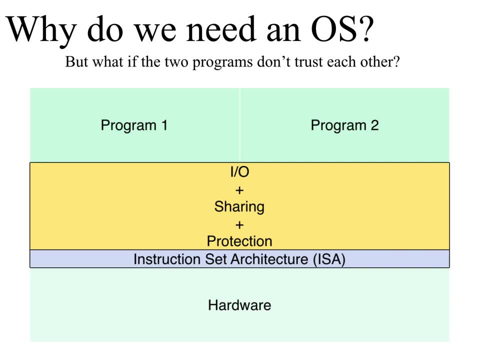 so that's another aspect of protection. and then sometimes you have to protect the hardware from the programs. some programs may not be allowed to, say, access certain hardware devices, say like the microphone or your camera. so who itself? well, again, that's the role of the operating system and sometimes these. 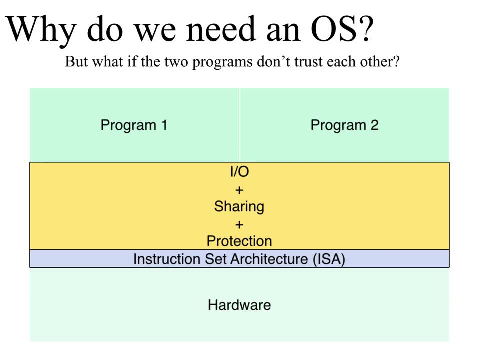 programs may not trust the hardware. you might have malicious hardware on a computer that might affect the software program. so again, operating system plays a role here, there, where it might protect user programs from untrusted hardware. so, as you can see, a prediction can be interpreted in many different ways, and 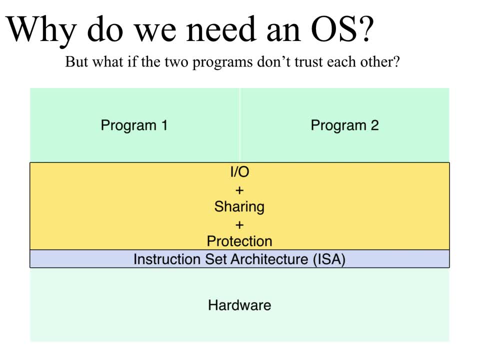 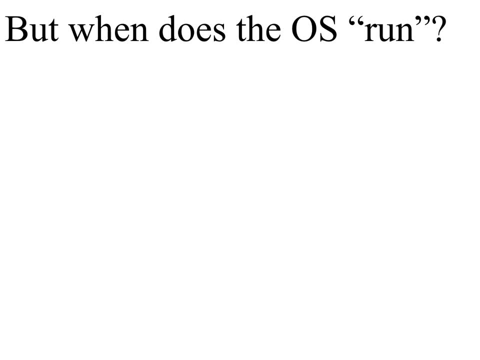 and of OS has a key role to play in all of these situations. all right, so now we know that OS has three primary roles, which is to manage IO, to do multiplexing or sharing, and then to provide protection. but when does the OS do all these things? in other words, when does it run on the CPU? 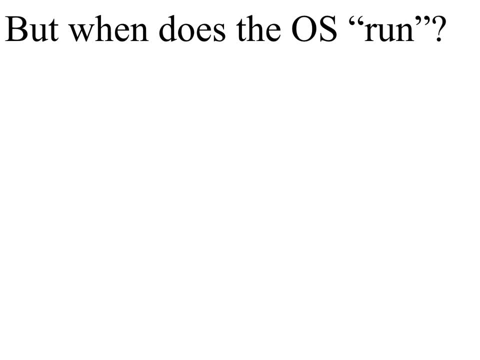 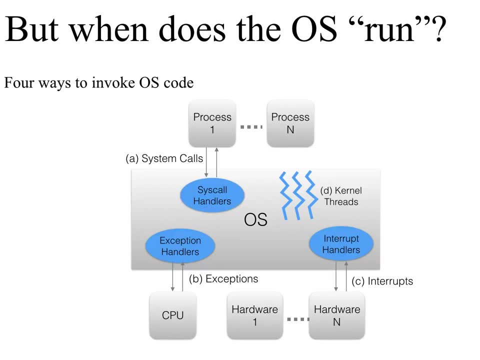 you? under what situations does it run? so, if you think about it, once an operating system boots up and during the normal execution of of your computer, there are a few events upon which operating systems code could execute. so I stress upon the word, even because I'm 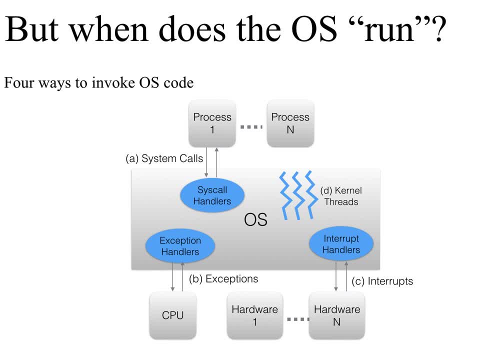 saying, implying that the operating system doesn't run all the time and it normally runs in response to some events. so what can these events be? well, the most common event is that, let's say you are running a normal user level program. the program needs some special service from the operating system, like 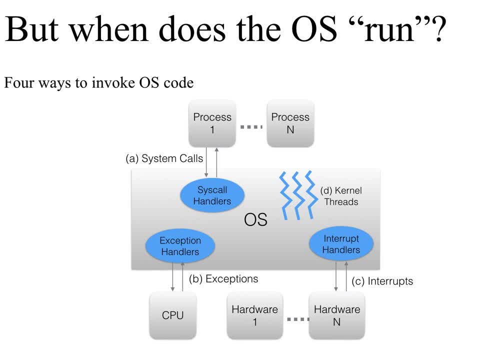 accessing the file system or communicating over the network. in this case, the process would make something called a system call. it's like a request to the operating system and when the system call is detected by this processor, the CPU, the corresponding instruction is detected, then the CPU would switch. 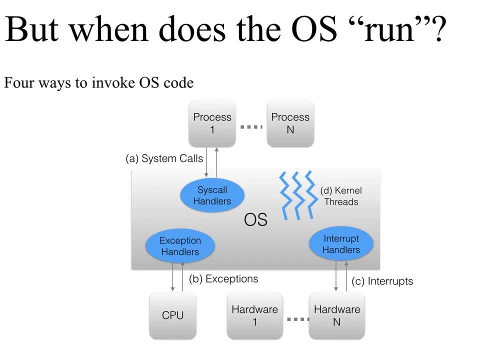 control to a piece of code that handles that system call in the operating system. so so a very common way to invoke system, the operating system code, is through system call requests from user level processes to the OS. the other reason the operating system code could execute is due to exceptions, the by exceptions we mean that when it 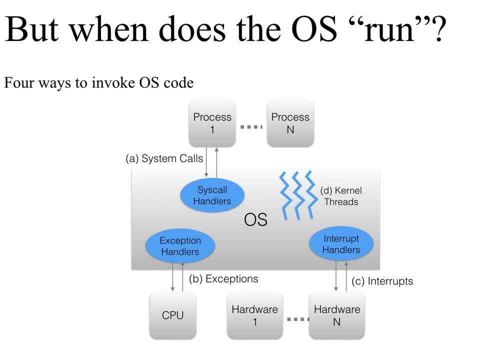 normal user level program, it does something that's usually wrong or incorrect, for example, a null pointer, dereferencing or divide by zero, or floating point exception or segmentation for access to invalid memory locations. so so these things are exceptions or errors that must be handled by the operating system. so in this case the processor will again. 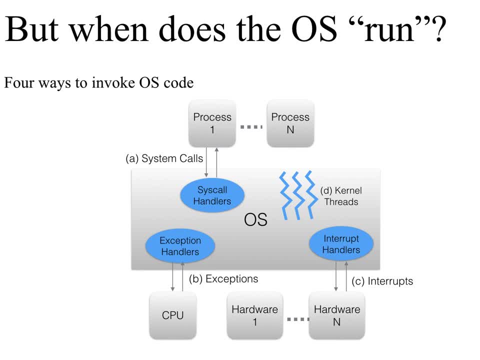 jump to into operating systems code somewhere in memory, which will then handle the error and and take appropriate actions, such as killing the process if there was a malicious action by the process. the other common reason why os code would execute is because of hardware interrupts. so this is interesting: that hardware can actually invoke os code. and how can it do that? by sending interrupts. 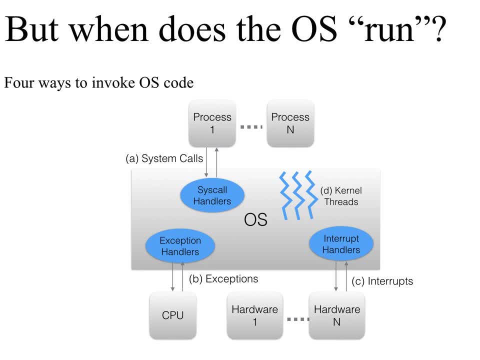 to the cpu. so whenever hardware has an event to handle- for example a network card receives a packet that has to be delivered to the os and then and then to some process- so the network card would send a hardware interrupt to the cpu, which would then jump to some piece of os code which would 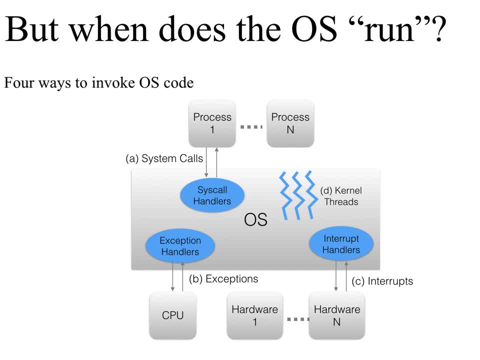 handle that network interrupt or a network interrupt handler. so for different types of hardware devices you can have different interrupt handlers in the os and the cpu. so these interrupt handlers are sitting there in memory waiting for the event to occur and whenever the event occurred they get invoked, just like normal functions get invoked by a process. 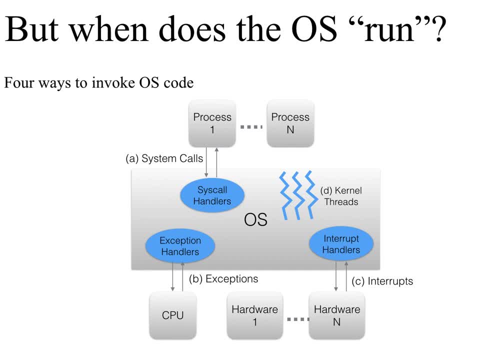 right. so all these three mechanisms we have discussed, they are in response to certain events- the os doesn't run all the time- and in certain events occurs system calls or exceptions or interrupts, the corresponding functions in the os get invoked. and then there is a fourth mechanism where, which is 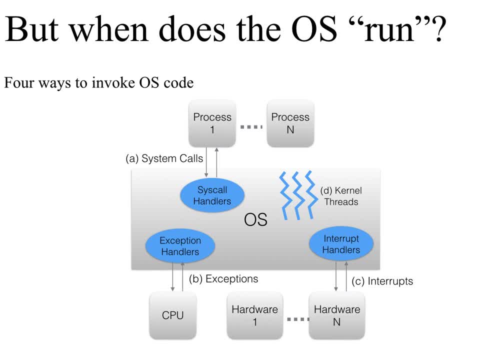 like traditional processes here the os, after booting up it can start a bunch of persistent threads or kernel threads. these execute regularly, periodically maybe, or maybe in response to certain events, but rest of the time they are in blocked state. for example, you might have some kernel thread to record all the events, all the critical. 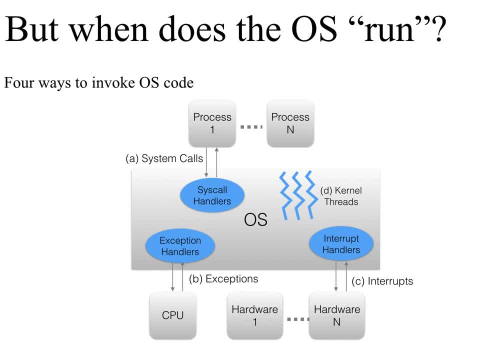 events in the system, like system log demons, and these might execute as kernel threads the most of the time they are sleeping and occasionally they get woken up and executed as kernel threads. so these are the four different ways, uh, in which os code could uh get invoked or or run, as you may call it loosely? 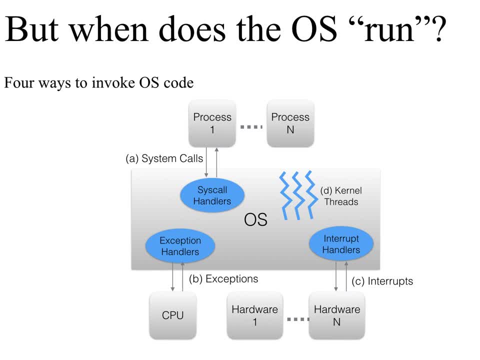 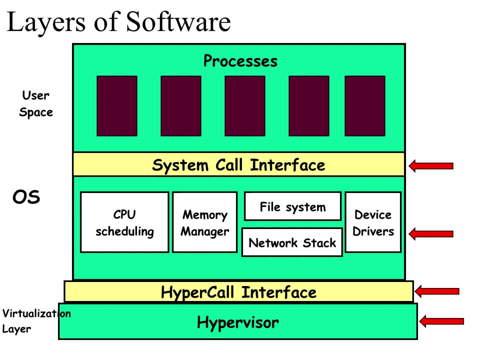 system calls exceptions, interrupts and as long-running kernel threads. so here's another view of the various layers of software that we have discussed so far. we have talked about processes that are normal user level programs, and then we talked about the operating system, which consists of various cyst software components for performing i o, for doing multiplexing and for prediction. 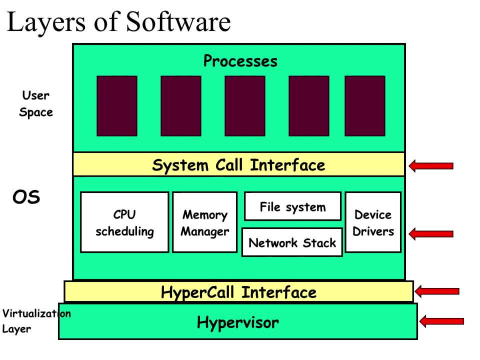 and then processes can talk to the to the operating system through the system call interface. there is special requests to the operating system to execute certain privileged operations on behalf of processes, and then normally an OS would directly interact with the underlying hardware through the instruction set architecture. but 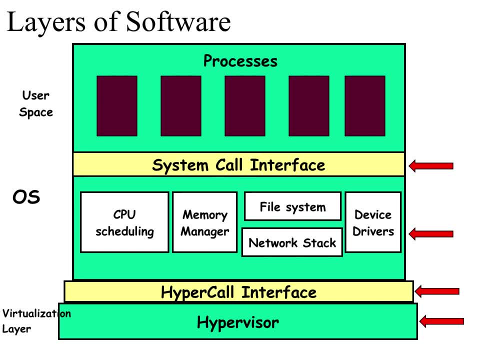 increasingly. what we are seeing is another layer of software between the traditional operating systems and the hardware, and this software is called the hypervisor, which provides a functionality called virtualization. so what that usually means for most people is that you would be able to run multiple instances of different operating systems side-by-side on the 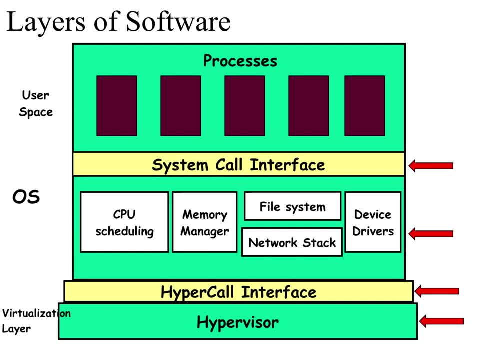 same hardware. so hypervisor is like an operating system for operating systems and most of the time hypervisor tries to stay transparent, meaning invisible, unlike operating system, which makes itself visible to processes through a system, call interface, a process, know there's an OS and they can request certain operations to the OS through 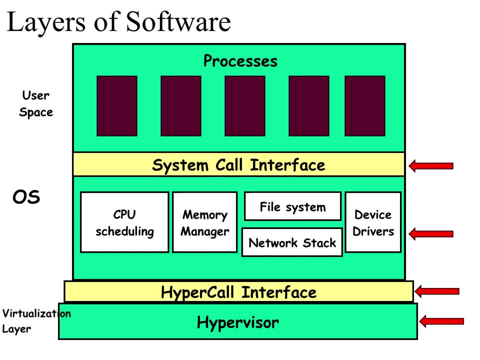 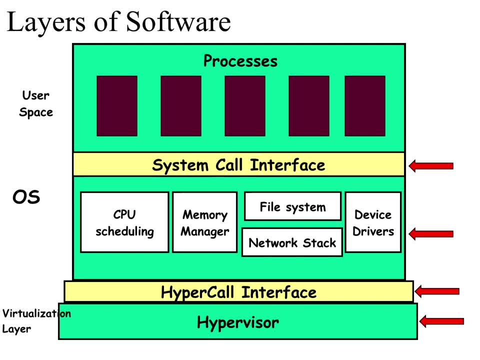 its actions, intercepting certain privileged instructions, emulating them and so forth. in certain situations, the hypervisor, for performance reasons, the hypervisor may choose to make itself visible to the OS and in order to do so, there is, there, can there might be a hyper call interface between the OS and. 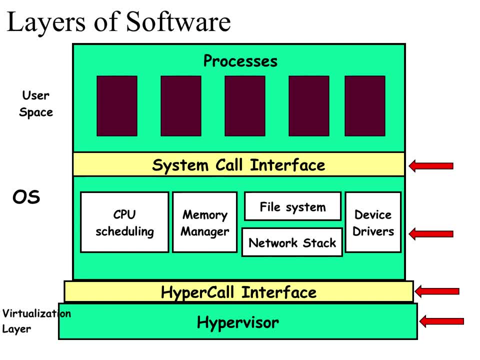 the hypervisor. just like there's a system call interface between process and OS, operating systems can use hyper calls to more efficiently request certain services from the hypervisor. so we will talk more about virtualization later in the class, but also touch upon aspects of virtualization and hypervisor as we 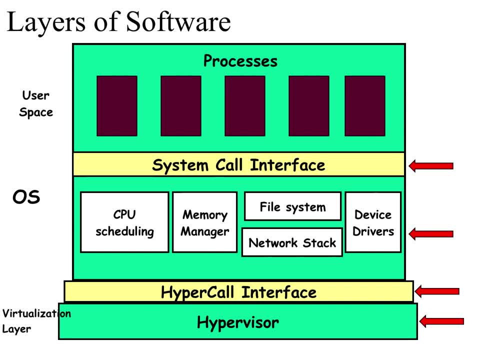 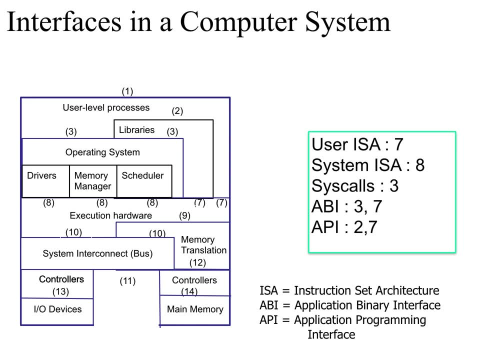 discuss other OS components. so in this slide I want you to look a little deeper into the various interfaces available in the entire computer system, from the hardware all the way up to the software. so if you look at this picture, this picture shows the hardware- software interface which is right in the middle. 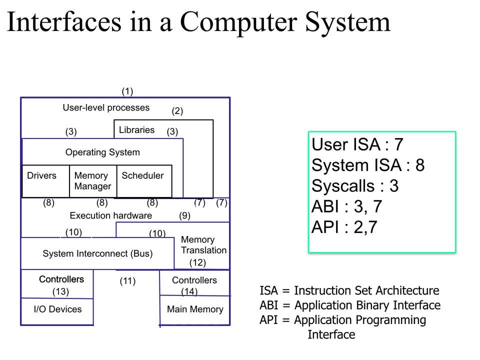 labeled seven and eight. as we discussed earlier, this hardware software interface is called the instruction set architecture, or ISA. everything below that line is hardware, everything about that line is software. now, within the ISA, you can see that it is. there is classified under two categories. the one part labeled seven is the user ISA or user instruction set architecture, which 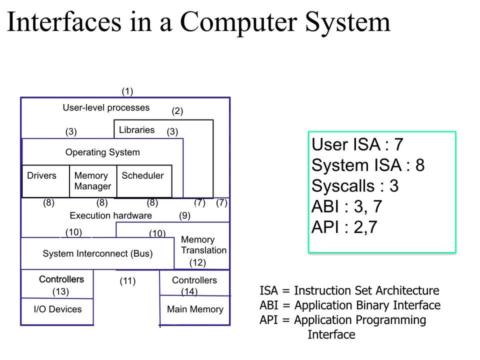 refers to instructions that normal user level unprivileged programs can execute on the CPU without any intervention by the OS, without having to request permission from the OS. so these unprivileged instructions could be doing load and store to accessible parts of memory, or doing normal arithmetic operations or floor. 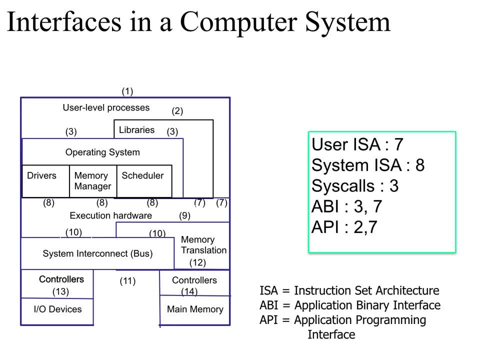 loading point operations and so forth. and then the system ISA instructions are special instructions that provide privileged access to the underlying hardware. so because these provide privileged access to the hardware, only the operating system is allowed to execute these instructions. that's why it's called the system ISA. so normal user level programs would execute the 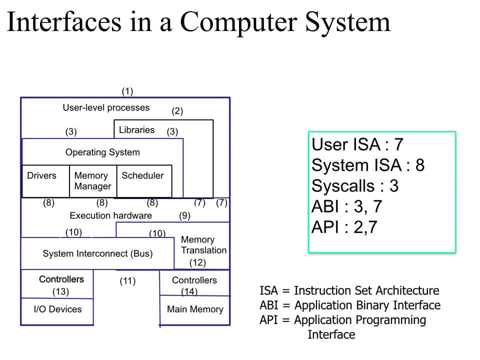 user ISA instructions to execute on the CPU most, or and then when they need special services from the OS, they would invoke system calls. the system call interface, as you can see, is labeled three in this picture, and the OS would then execute privileged instructions to service the corresponding system calls. so, looking down at the hardware level, you can see. 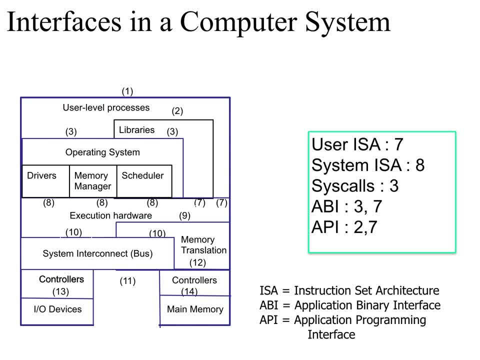 there are various components in hardware again connected to each other through hardware level interfaces. for example, the execution hardware or the processor and its registers forms the main interface between hardware and software. below the below that, you would see that there are IO devices at one end and main. 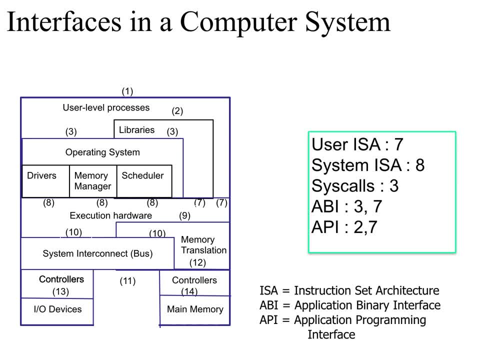 memory or the DRAM at the other end. so everything else in between is meant to have the CPU, I devices and main memory interact with each other. so what that means is that the CPU, might, you might- issue instructions to IO devices to transfer data. so for that there is a 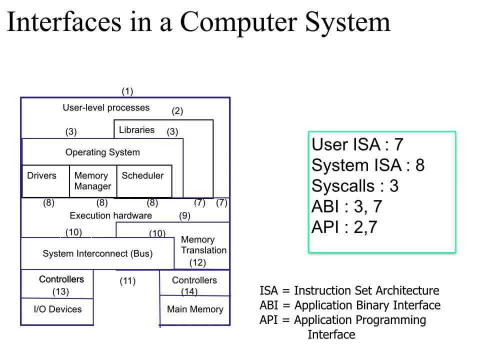 system interconnect bus which carries data between the CPU and IO devices, but then the system interconnect bus may also enable the CPU to talk to the main memory through memory controllers and memory translation units in, and then the main memory and IO devices may also directly talk to each other through the 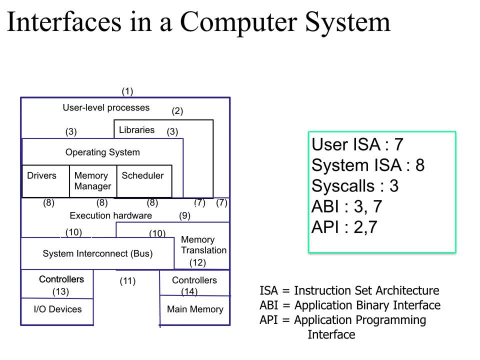 system interconnect bus. so, as you can see from this picture, the system interconnect bus, or the system bus, plays a really important role in moving data and commands around between various hardware components. so the speed of the system interconnect bus is often really important for very high throughput, low latency data movement. so normally, system 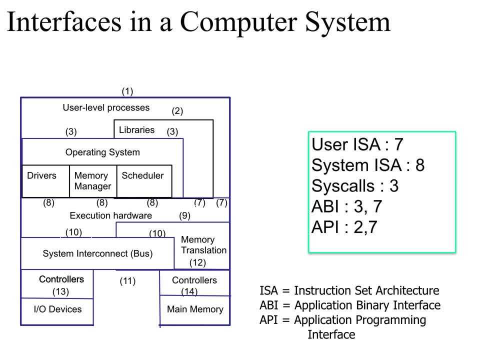 interconnect bus is more complex than what's shown in this picture. there are many system buses, some for high-speed devices and some for low speed devices and so on. so we are not going to go deeper into the hardware component, but it's important to keep this picture in mind as we discuss rest of the OS. 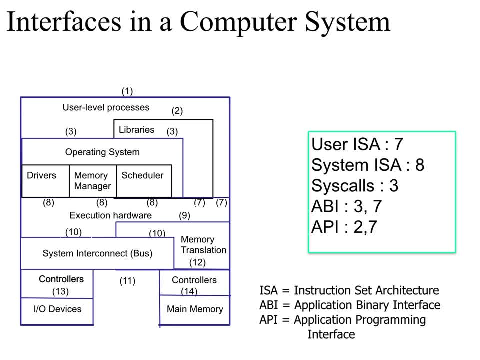 functionality. the one last thing I want to point out is that a combination of various interfaces is a naturalě inter-connective interface which will enable your hardware to know how to connect the system to another interface. we have seen that for a while now, but the human interface is one of the most common interfaces in this world, which is proxy-based, is a complex interface and therefore you have to connect to multiple interfaces: the data center interface, the data center interface, the system and normal devices, the system and normal application, the CPU, the GPU, the chip, the GPU, the CPU, the CPU, the GPU, etc. 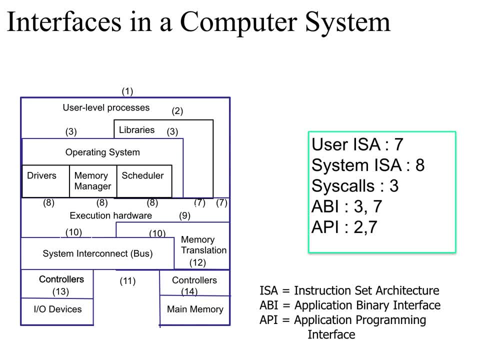 interfaces have important roles to play in what the operating system does. so we already discussed the ISA, or the instruction set architecture. you can take a combination of the user ISA, which is number seven, and system calls, which is numbers three, and if you look at this boundary formed by interface, number three- 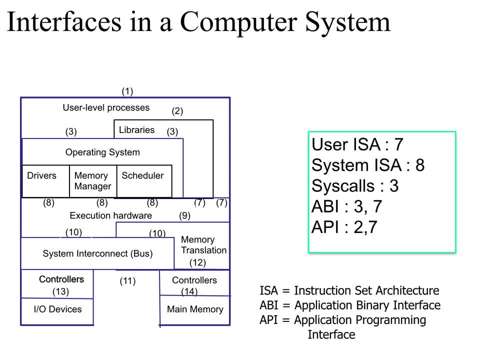 and interface number seven. this has a specific name, called the ABI or application binary interface. what this means is that the ABI is the view of the rest of the computer system as seen by user level processes. whatever user level processes do, they are either executing user ISA instructions directly on the 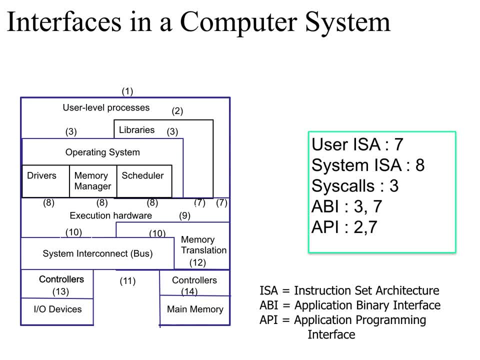 processor or they are executing system call instructions which then transfer control to the OS to do something on their behalf. so ABI is really important for portability of processes. so if you look at the ABI you can see that the programs, because if you take a binary executable and move it to a computer, 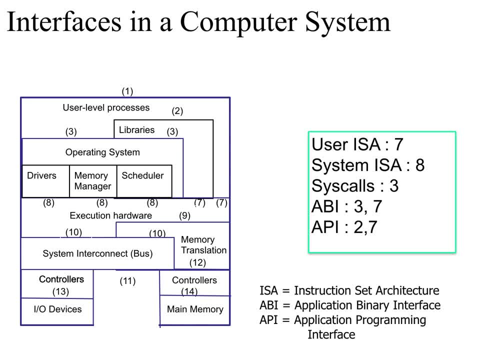 which has a different ABI, say different user ISA or a different system call interface, then the program won't work right. so ABI is really important for portability of binary executables. that's why if you say, take an executable that's compiled for on Linux operating system and move it to, say, an identical, 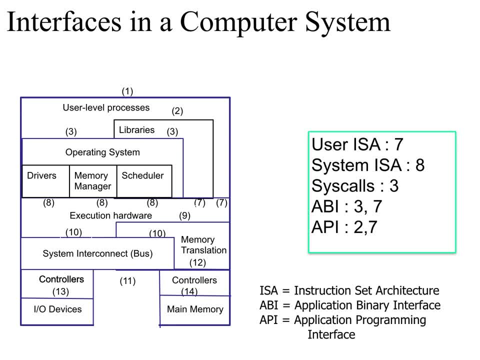 hardware but which is running to a Windows operating system, then your same executable won't work, even though maybe the processor is to like SATA 6 processor. so what that means is the system call interface for Linux and Windows are different, so the ABI is different, so your executable is not. 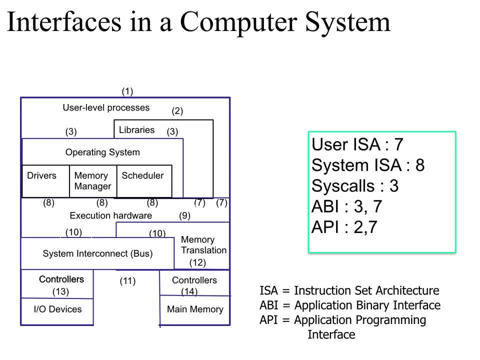 portable anymore. the other interface that you might want to understand also is API, or application programmer interface. this consists of another interface labeled number two for libraries. so when you, as a programmer, you write code, then you are using certain libraries which provide certain functions that are written ahead of time for you to use just to make your 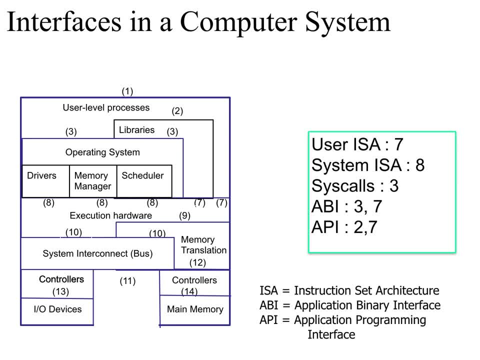 life easier. so these functions either get statically compiled into your program or they get dynamically linked into the program at runtime. and and these are, these are still user level pieces of code. so, as well as programmer is concerned, the programmer needs to know this combination of interface which is two and seven, which is what user level user is. instructions to: 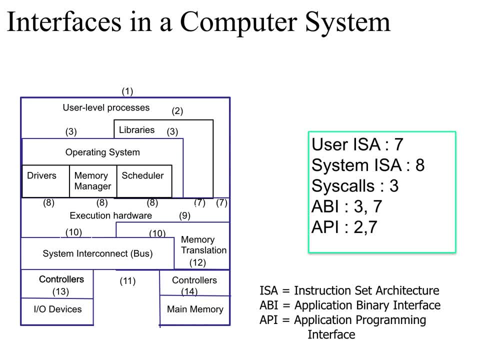 execute and what library routines to invoke. but once the program is compiled and are linked, then you don't actually deal with the interface number two: so so programmer has to know API, but during runtime API is more important. so API is for programming time and ABI is for runtime. 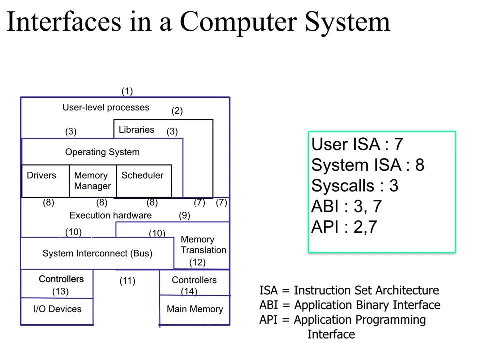 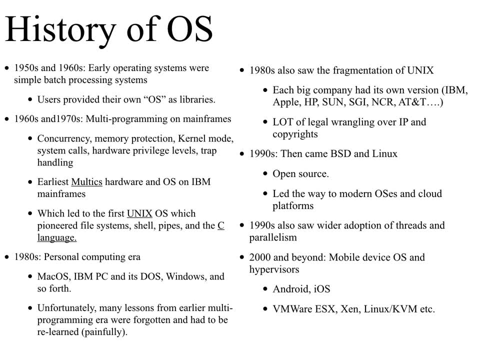 right. so this brings us, finally, to a brief history of operating system, and it turns out the history of OS is really interesting, just like, you know, any other history of computing technology. so when computers started becoming mainstream around 1950s and 60s, these were mostly large mainframe computers. 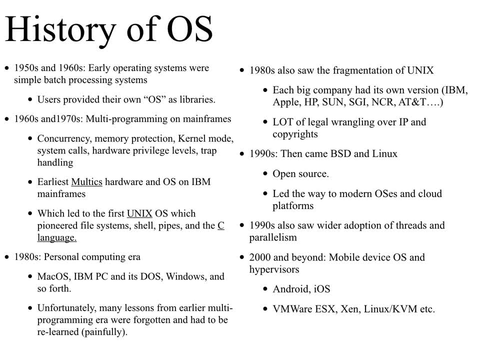 these were batch processing systems. it would feed in a job, the computer would just do that one job at a time and then, when it's done, it would pick up the next job. so users would provide their own operating systems as libraries that we discussed earlier, to know how to interact with the hardware. and- and there 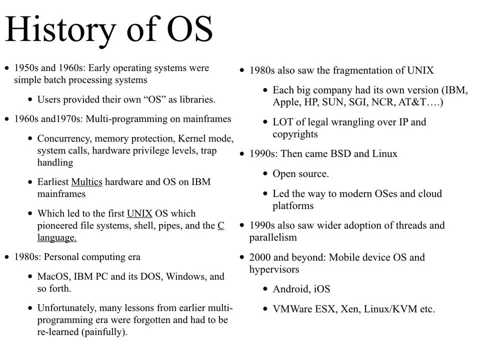 was no multiplexing or protection issues in the in the RDS computers. as time went on, there was a need for multiple programs to be running simultaneously or concurrently, so multi programming requirements led to addressing issues of hardware sharing, which meant that you had to bring in notions of concurrency. 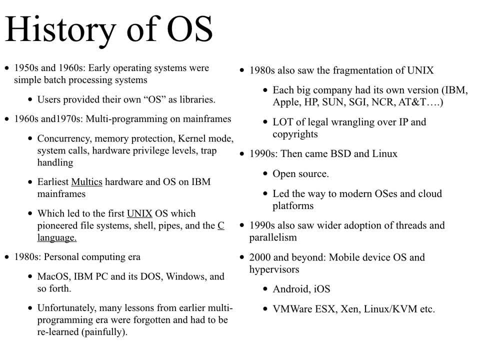 memory protection, formalize what it means to be an operating system, provide system call interfaces. and the hardware had to distinguish the privilege levels between the hardware and the hardware and the hardware had to distinguish the between the OS and user level program. so hardware provided this notion of a 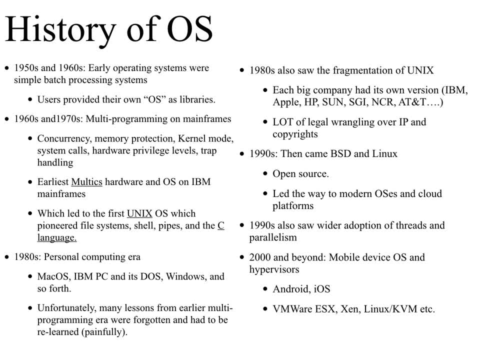 privilege level in base for the OS to control privilege level transitions and trap handling, meaning for exception handling or interrupt handling, and so on. this was one of the pioneering hardware in the early days was the multics system, which was both which had innovations in both the operating system and the 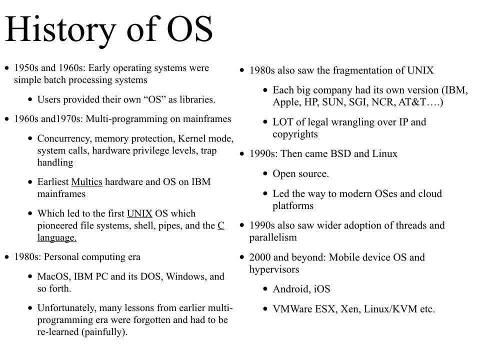 hardware. that led to the development of the Unix operating system, which addressed many of the drawbacks of multics- multics itself. it was pioneering. but then Unix went further and introduced the notion of file system as a central organizing concept for all hardware and system resources. so Unix also introduced the C programming language, which is a fairly 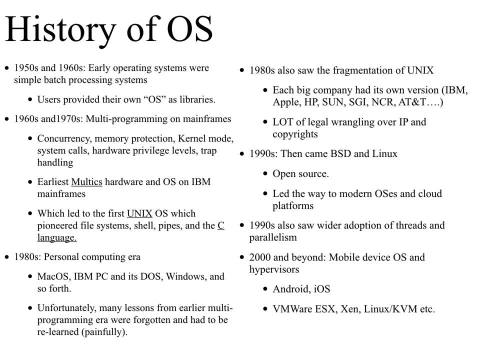 dominant programming language. even today and then in the 1980s people wanted computer running software to be able to run computer running software in the computer right on their desks. so that led to personal computing era and a lot of personal computers such as the Mac computer, the IBM PC and and, of course, 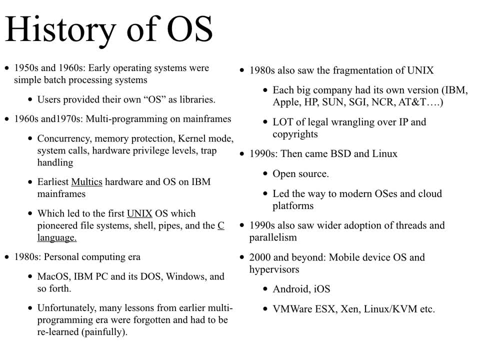 the Windows and DOS operating systems came forth. unfortunately, during this time, many of the lessons from the mainframe and in multi programming era were forgotten and there to be painfully relearned in. 1980s also saw wider adoption of Unix, but also a fragmentation of Unix into customized 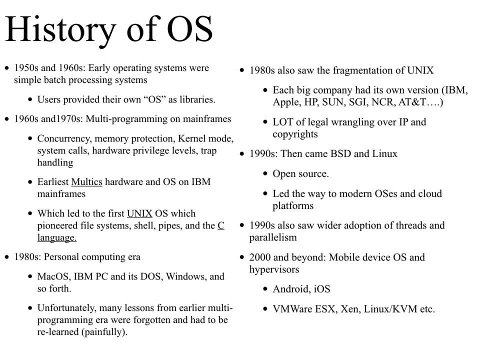 commercialized versions from different companies and this led to a lot of compatibility issues and and and fights over intellectual property and copyright and at the same time, open source movement was taking root and from that came operating systems such as free BSD and Linux and the other two systems that. 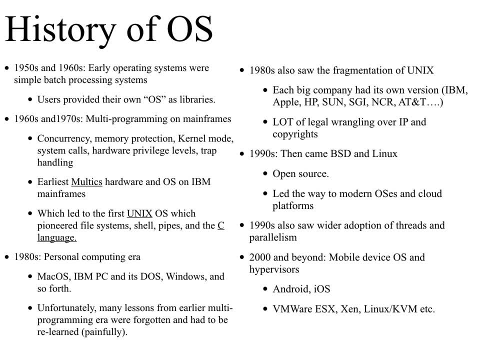 were developed in the 1990s and these kind of led the way in democratizing, in commoditizing operating systems. so it's also coincided with the rise of the internet and and, and together they have led to the computing landscape that we see. so in the 1990s was also very interesting in that, from the notion of processes, the use of 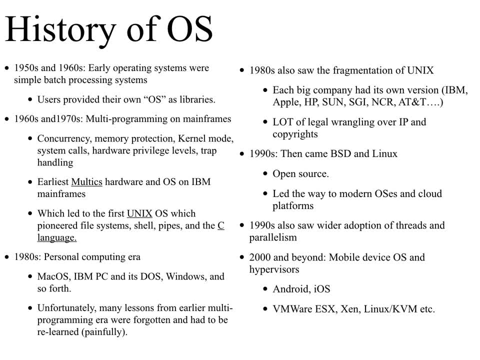 threads became more prominent, more mainstream, because now there were CPUs and being designed that were that had mud there, there were multiple CPUs to be handled and there were multi core CPUs that were coming out and and parallelism was becoming really important and operating systems had to be redesigned. 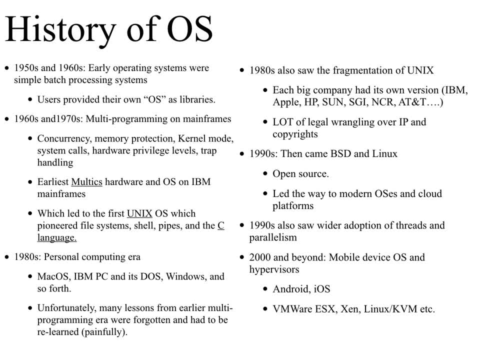 to handle parallelism and concurrency and higher performance requirements. so in in 2000 and and later the last 20 years, essentially cloud computing became very prominent as internet matured and and large data centers came up. at the same time, mobile devices, it is handled to, became very important and all these platforms 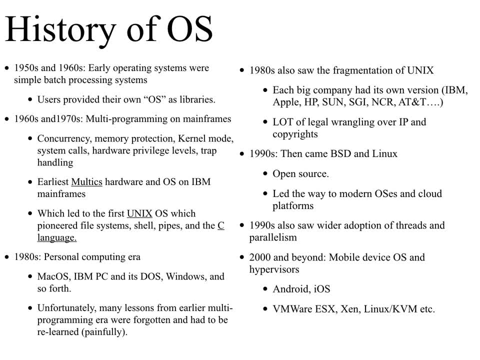 required operating systems. so the the traditional open source operating system such as Linux, are being adopted to run on these various platforms. so, for example, Android is a variant of Linux. iOS is again like a variant of Unix that descended from Apple's own version of operating systems. at the same time, we talked about hypervisors earlier, so